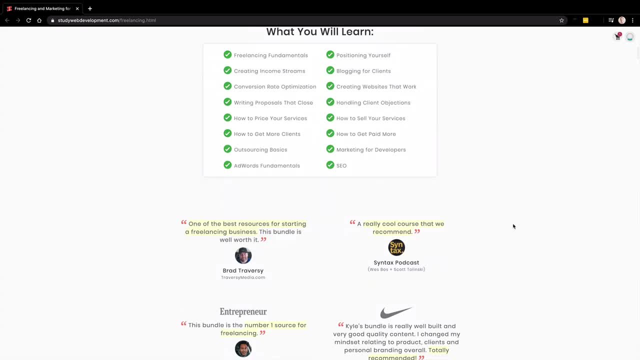 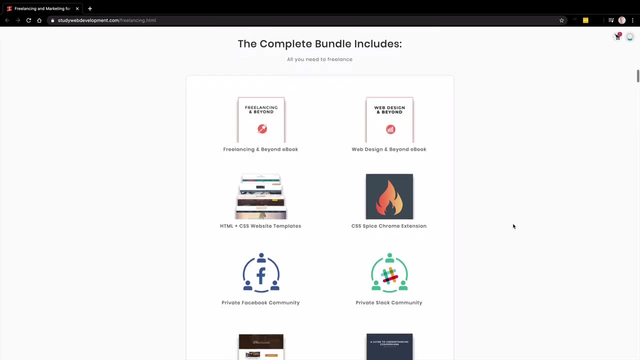 ability to create products, and you can do that for yourself or for other people, Whether you want to freelance part-time to earn some extra income or try to make this your full career. this bundle is going to have some great tips and templates and strategies for you to follow to go. 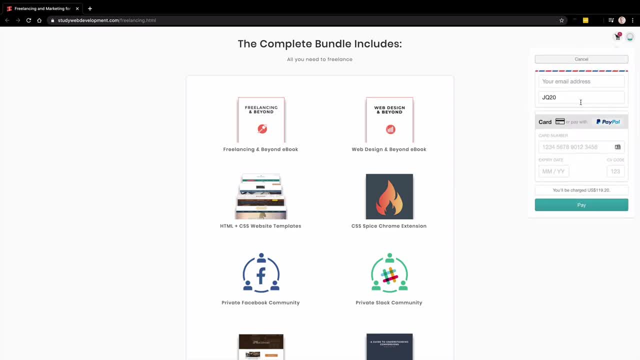 and build that clientele and grow your business. Now, if you're interested, check out the bundle and use the coupon code JQ20 to get 20% off the entire bundle. I think it will be well worth your time and you should definitely check it out to start your career as a freelancer, All right. 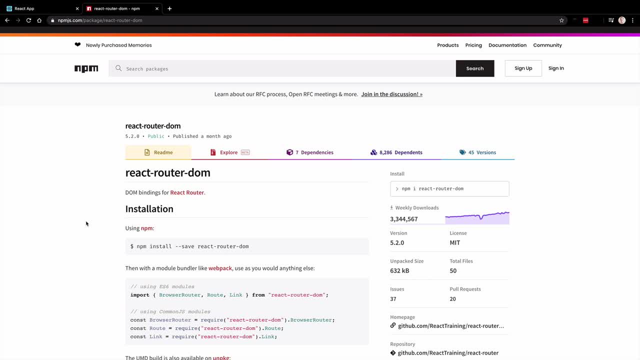 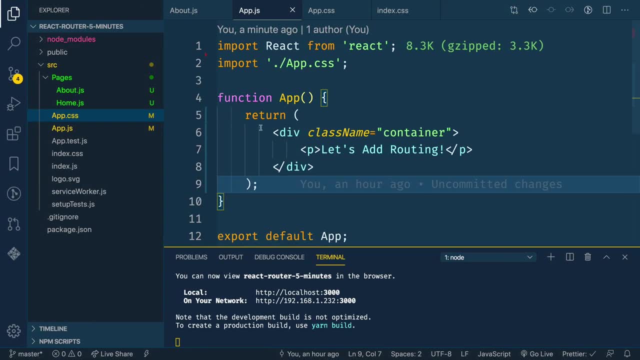 we're going to go ahead and set up React Router in five minutes here using this React Router DOM package from NPM, And first I just want to show you there's not really a whole lot going on. I've basically got a starter React application using Create React app. I took out all of the base stuff. 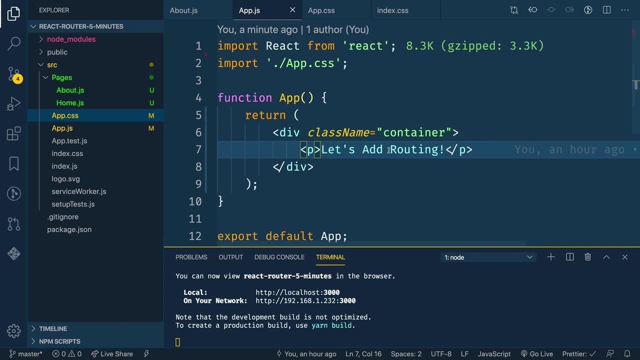 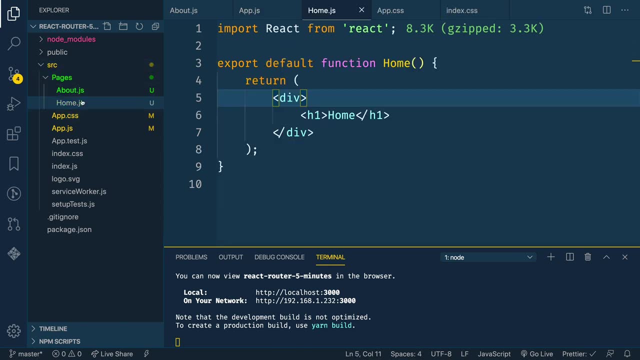 that I was going to show you. I'm going to show you how to set up React Router in five minutes. It's in the appjs. Just added a little paragraph tag here to say we will add routing. And then I've created a directory inside of source for pages And there's a home component which is really. 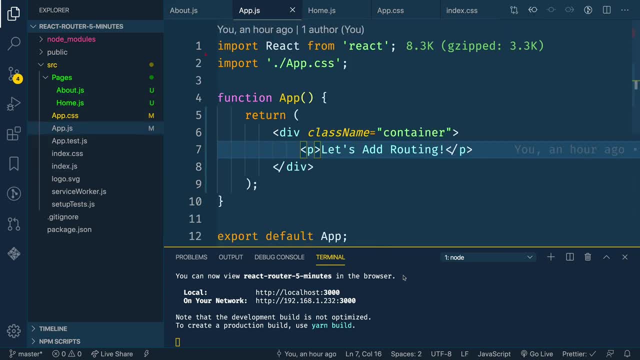 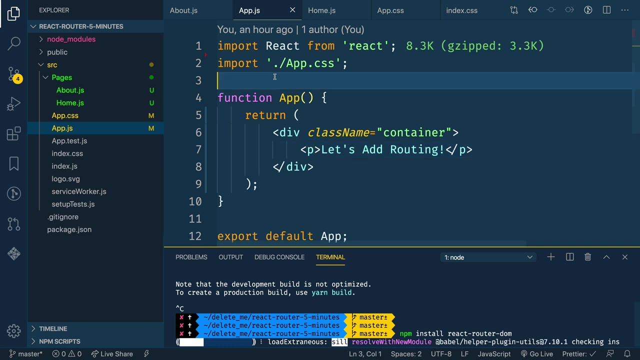 simple, obviously, and then an about component. So let's go ahead and let's stop the live server and let's install React Router DOM. So we'll install this package, And then there's a couple of things we're going to need to do. We're going to need to import the actual router into our appjs. 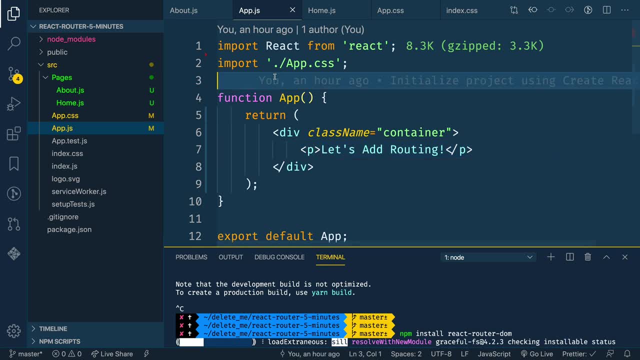 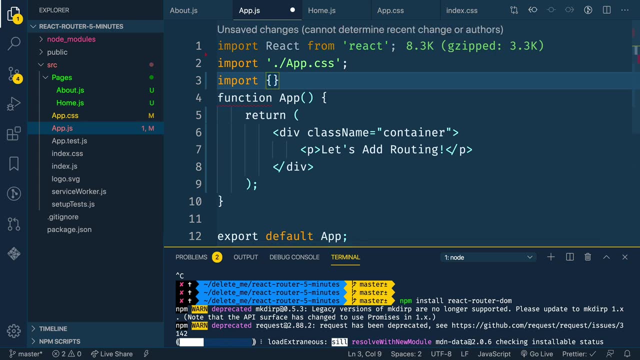 So, basically, what we're going to do is surround our app with the router and then conditionally display the pages based on which route the user is on. So what we'll want to do is do an import, And this will be fine. as soon as that package finishes installing, We're going to import route. 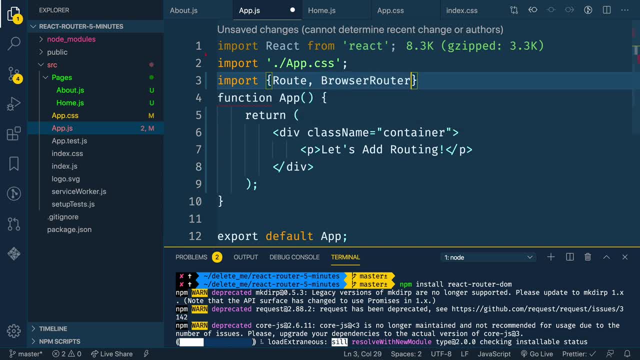 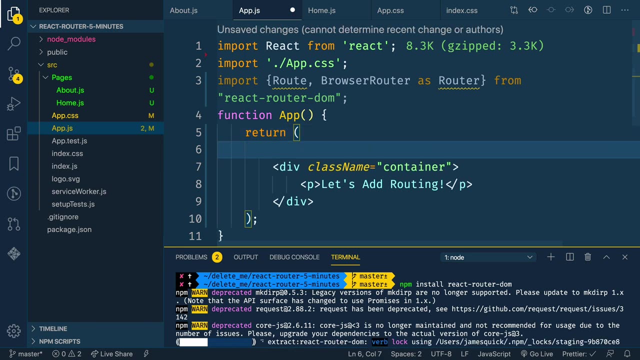 And then we're also going to import the browser router, And most people in most documentation I see they rename this a browser router as router And then we'll do that from React Router DOM. So with those things imported here now we want to wrap basically this entire container with our actual router. 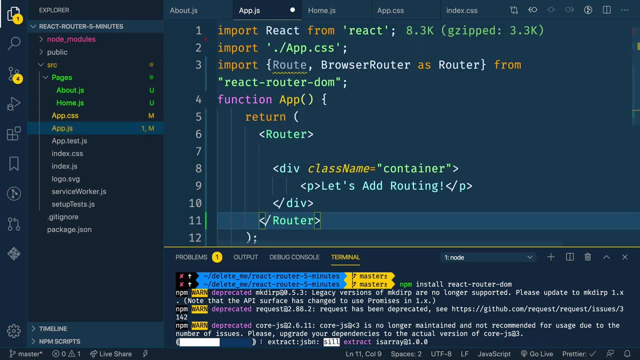 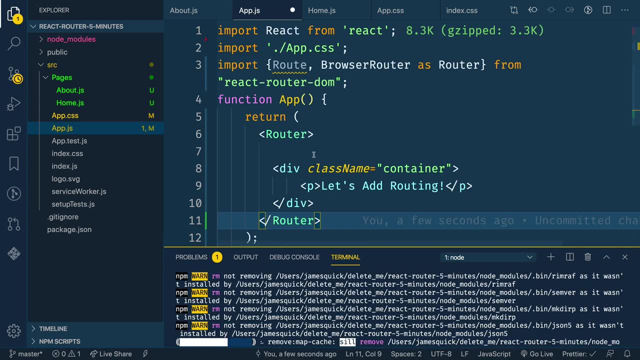 So we'll go ahead and surround this thing with our router And then what we want to do is have a place where we're actually going to put the different things that we want to display, So we can have those be our route. So if we have a route and then a path, each route will have two. 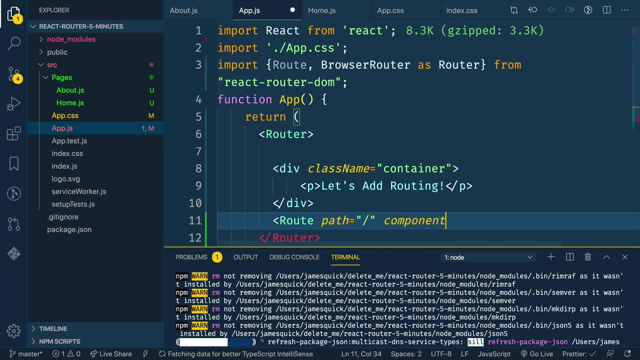 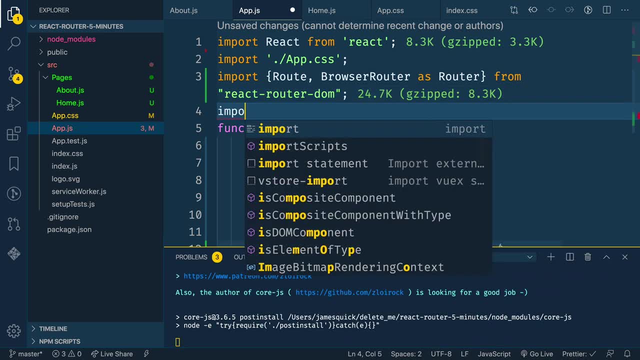 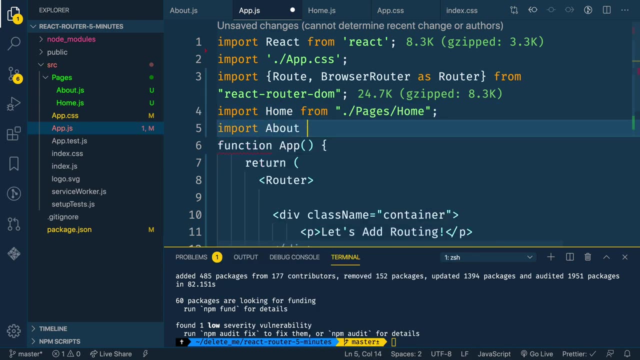 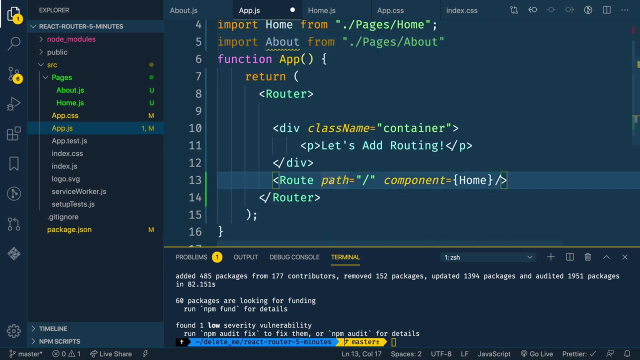 properties, a path, and this will be the route and a component, And in this case we'll have our home and about, So we'll import home from pages and then home, And then we'll do the same thing for about, So import about from pages, slash about, So I have both of those And we'll just create. 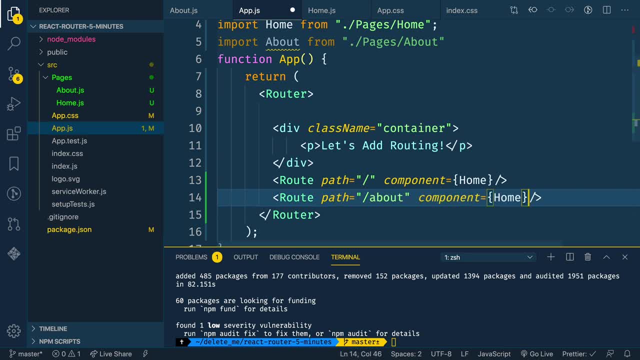 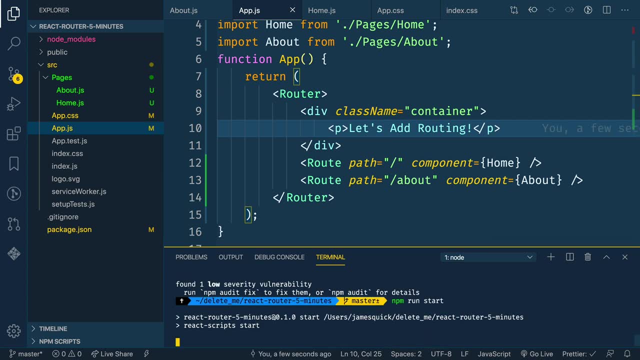 a new route here, So a second one for slash about and this should be the about page. Alright, so let's save that And then let's run npm, run, start again to start our live development server. We'll get this thing up and running here And hopefully, what we'll see. 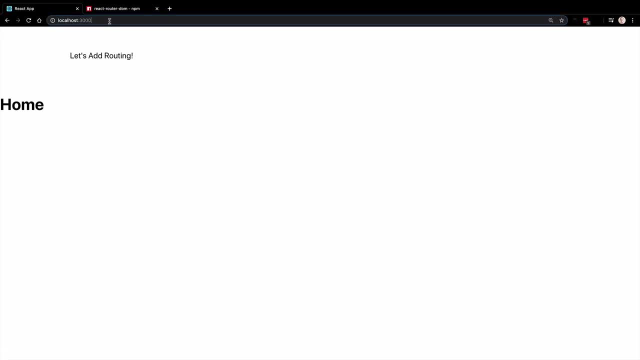 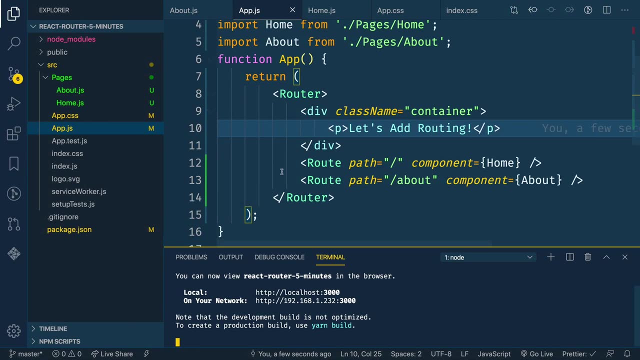 is that we see once this finishes loading, we see home And then if we come to slash about, we'll see something weird. It's about an home And the reason is this is a little bit odd, But basically the route path here is also a match for slash about. so when we have things that might 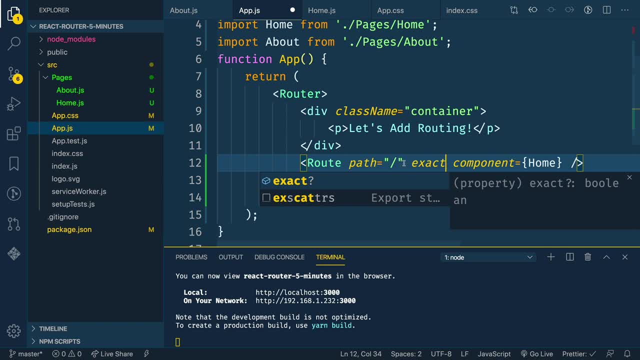 be sub routes of each other, we need to potentially mark them as exact. So what this means is only render this home component. So when we have things that might be sub routes of each other, we need to map them as an object If this, this path, matches exactly. so if it's just the slash and not 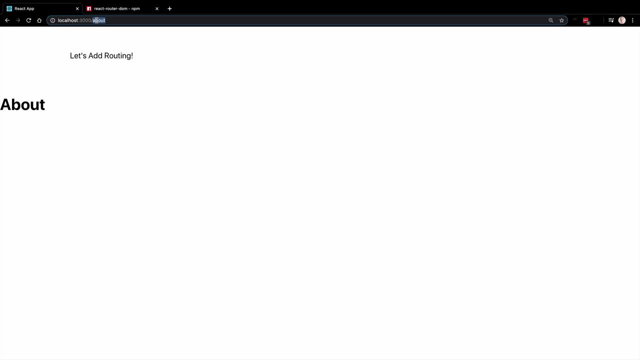 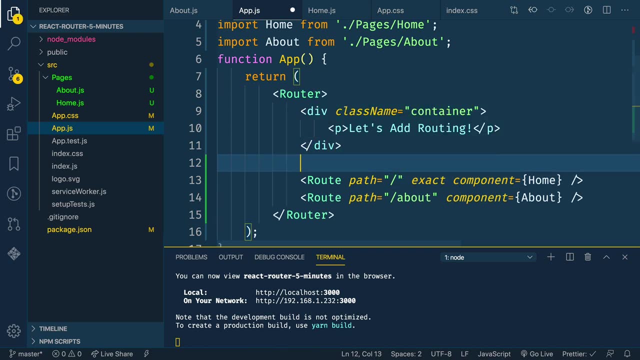 anything else. So if we come back now, we see there's the about And here's the index, which is our home. Now, if you wanted to solve this in a slightly different way, you can use a switch in react router So we can bring in the switch And with this we can wrap all of our routes. 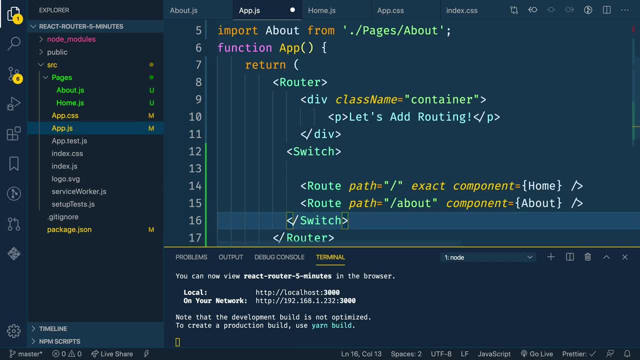 inside of a switch, switch here, And what this is going to do is it's only going to choose one of these paths. So we can get rid of that And then you'll see the path that you've made. But now we're going to want to render the path to be a cel, And then we don't have to render the path to be a cel. 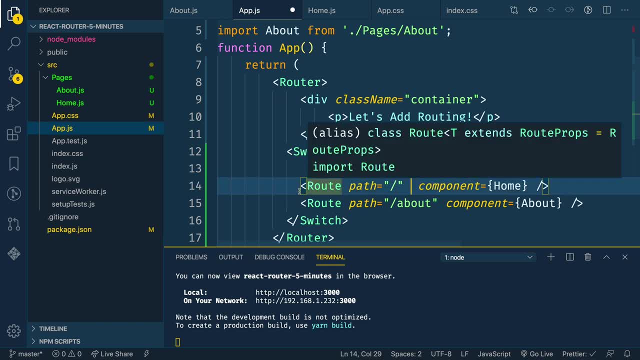 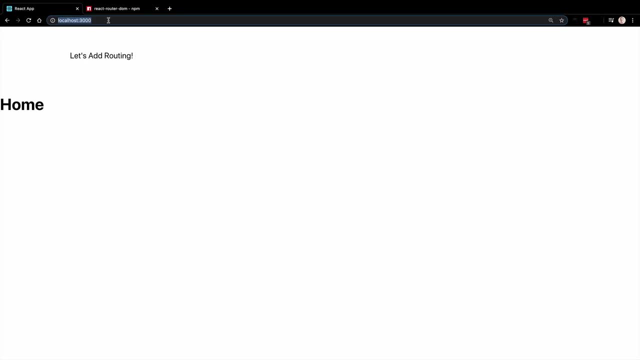 So we can get rid of exact, and then it's only going to choose one of these routes inside of here, So only one of those will show at a time and it'll be the first one that matches. So this will work, although it will be a little bit odd as well, because we come to slash about it. So it 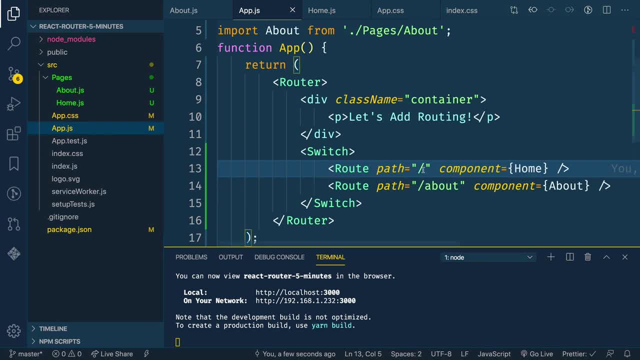 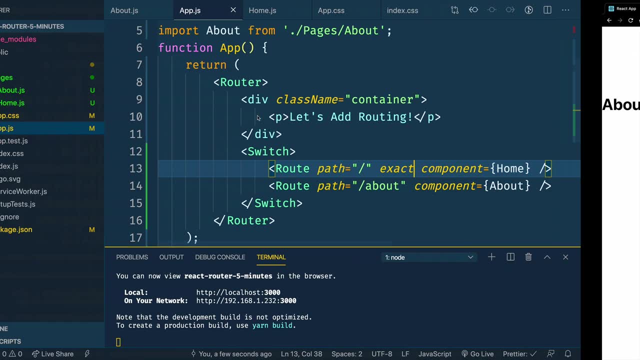 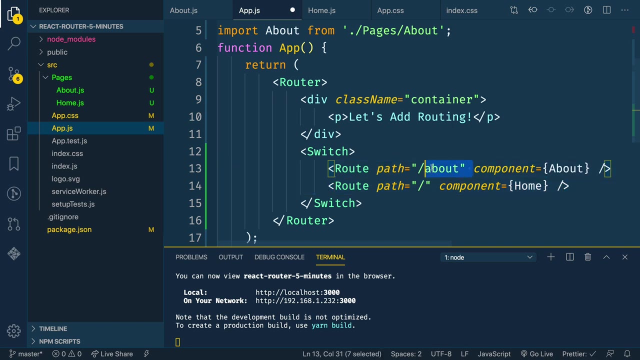 shows also slash home. Now this is again for the same reason that home also matches. So you could either mark this as exact again and now you'll see about, or you can mark this without the exact and then just have it come after the about. So basically, it's going to try to match this thing. 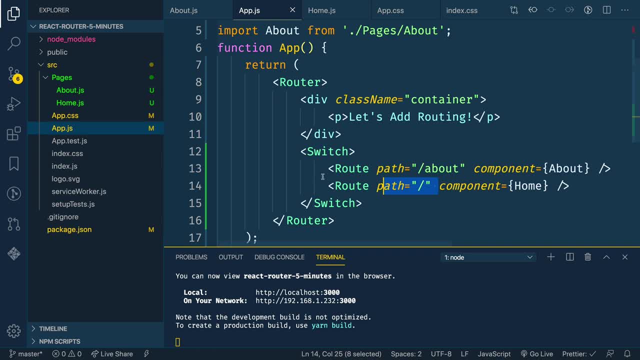 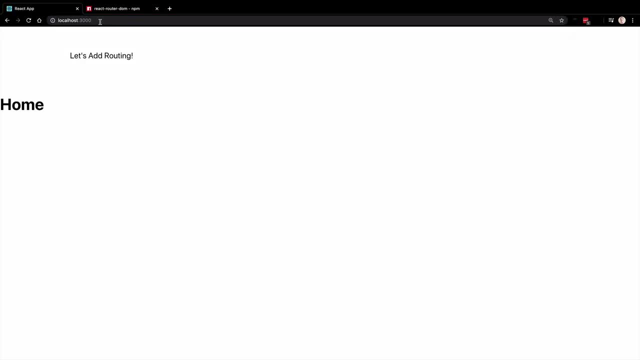 first, and if it matches it'll take that and then this one second. So here we should see the same thing. So that's using the switch there. So that's pretty cool, and if we come back home we should see the home page. And then, lastly, we can just add a little tiny nav here, just for testing. So let's do. 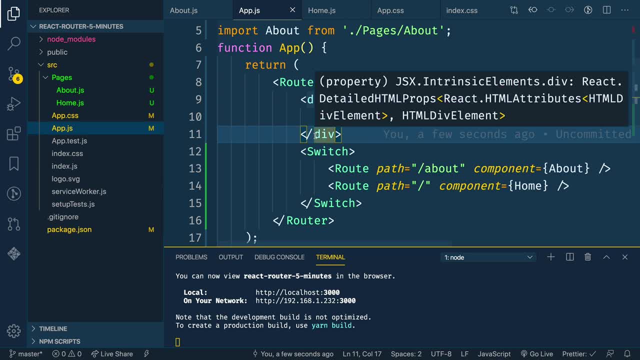 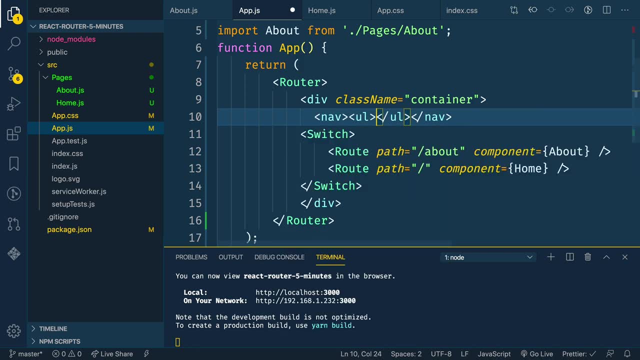 let's get rid of. actually, we could put all of this stuff inside of our container- and let's get rid of this and let's do a little bit of a nav and it'll have a ul and a couple of li items And what we want is each of. 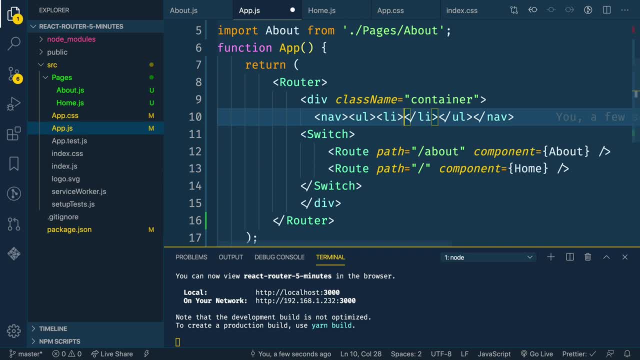 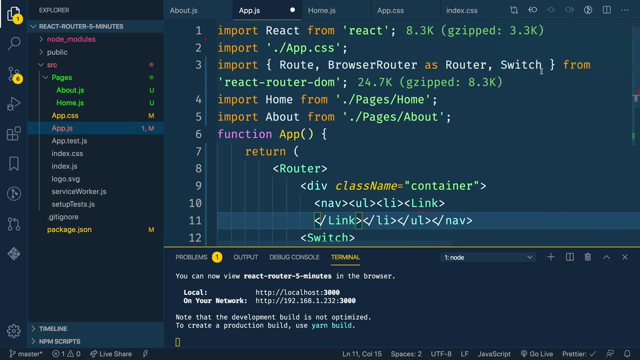 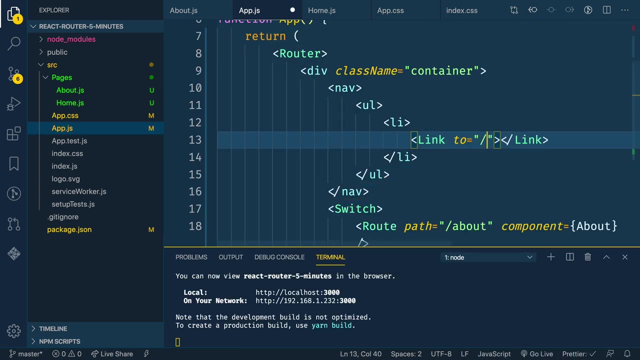 these to be links to the different pages. So actually, instead of or within the li, we'll have a link and we'll get some auto formatting here in a second, but we'll need to import the link here as well, And a link is going to have a property of a2.. So this will be. it's a slash and this will be. 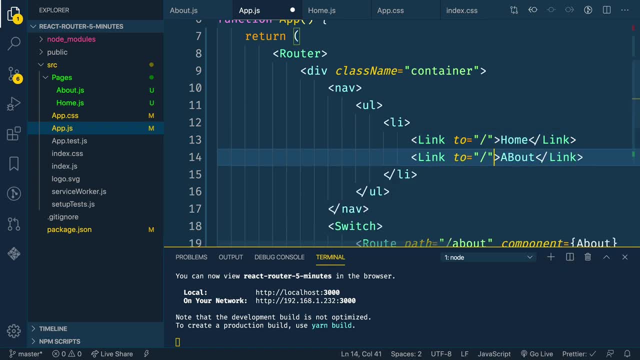 home and then we'll duplicate that and say about And slash about. Now the reason you want to use the link component from react router DOM is this will do client side routing. So if you just use your regular anchor tag with an href, it will actually reload the entire page with the link. 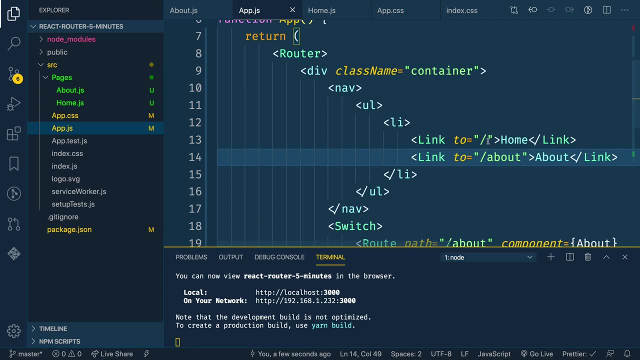 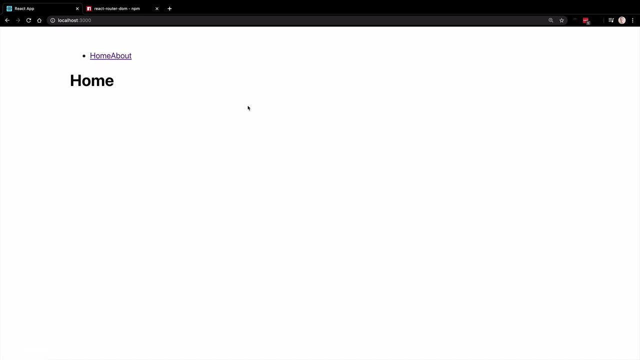 tag inside of react. These are going to use client side routing, so you're not reloading the entire application, You're just changing the page. So let's come back over and you see, I've got our two links. They look. maybe these aren't. 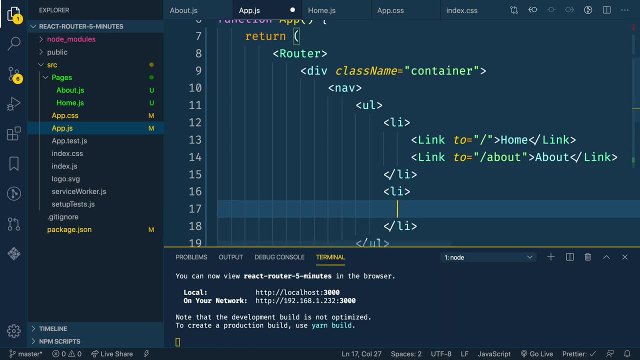 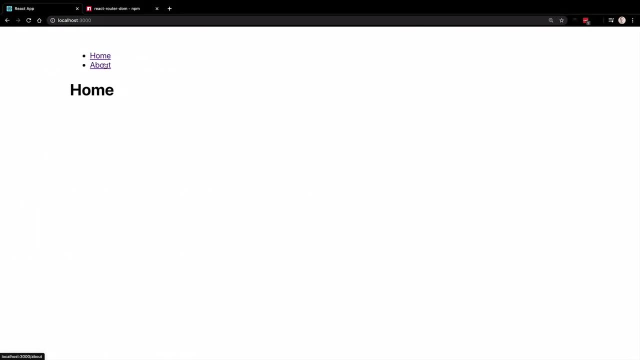 formatted correctly and they're not, because this other one should go. I'm going to take a look at how I'm going to create a couple of links here. So we've got the round inside of an Li and this is obviously not going to look very good, but just to show you how to set this up, we've got our homepage. 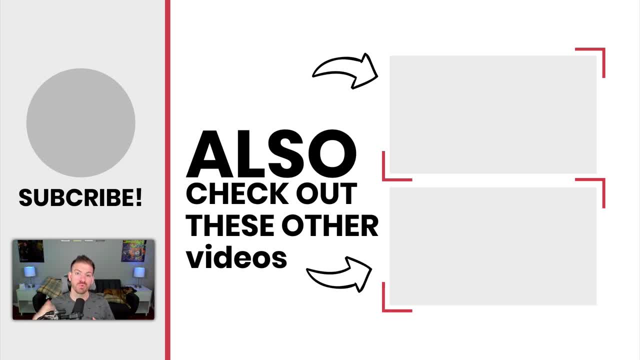 in about five minutes. here We talked about the browser router, renaming that thing to a router to wrap everything in our appjs: creating the individual routes, using a switch to be able to choose between different routes, and then using a link for client side routing as well. 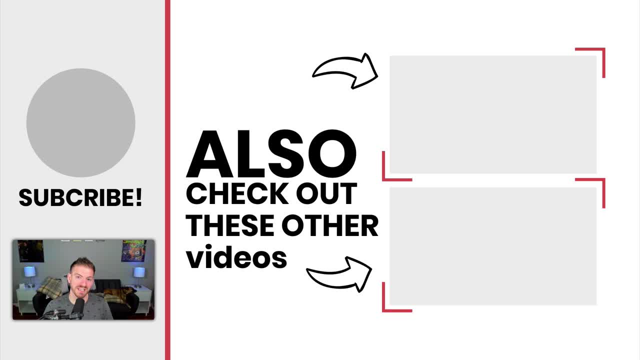 I really needed this as a reference for myself. Hopefully this is a really quick and nice reference for you going forward as well. Hope you enjoyed the video and I'll see you in the next one.